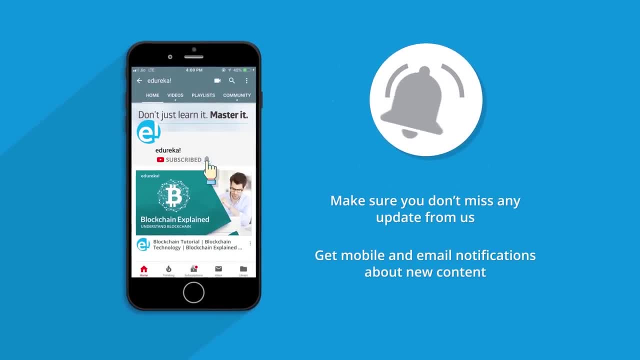 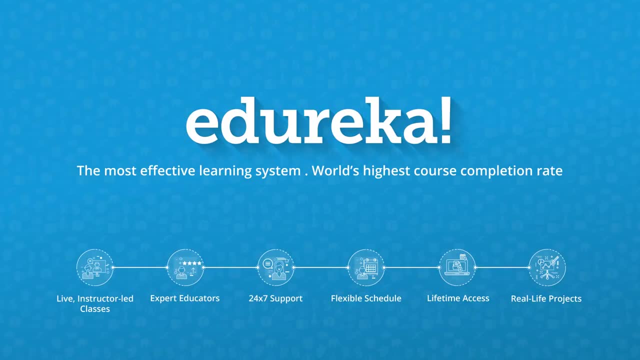 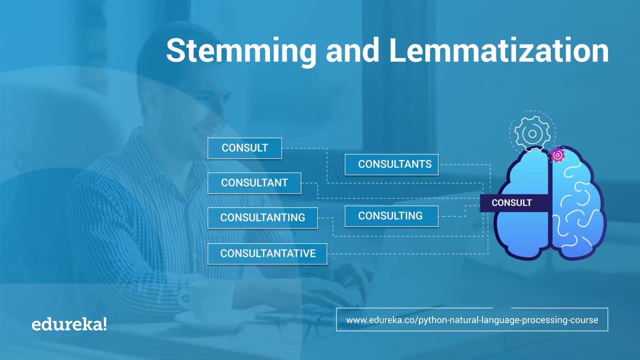 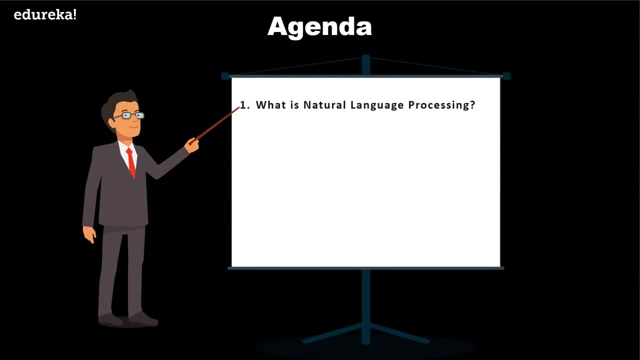 Hi everyone, this is Shainthini from Edureka, and in today's session we will talk about stemming and lemmatization. So before we begin the session, let's have a look at today's agenda. So we will start with the definition of natural language processing and then move on and have a 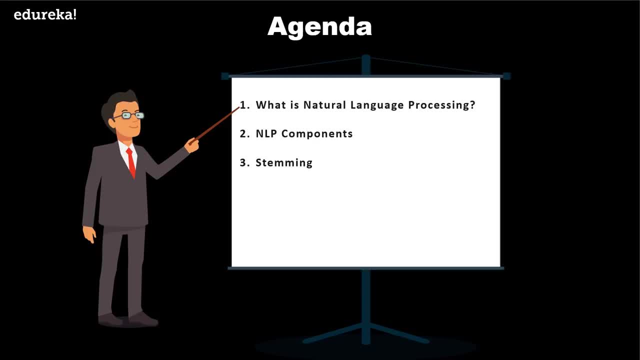 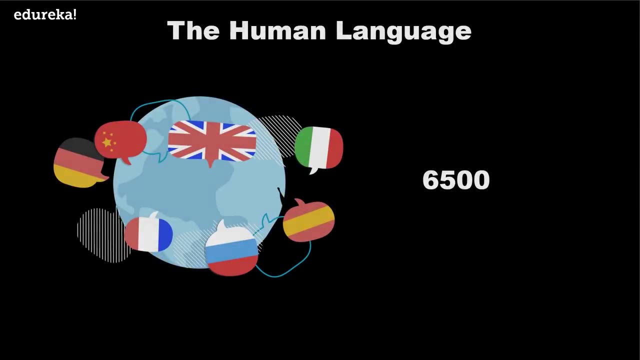 look at the components of NLP Further, we will see what is stemming and what is lemmatization. Moving on, we will also have a look at some of the applications of stemming and lemmatization. Finally, we will wrap this session with the differences between the two, So let's begin. 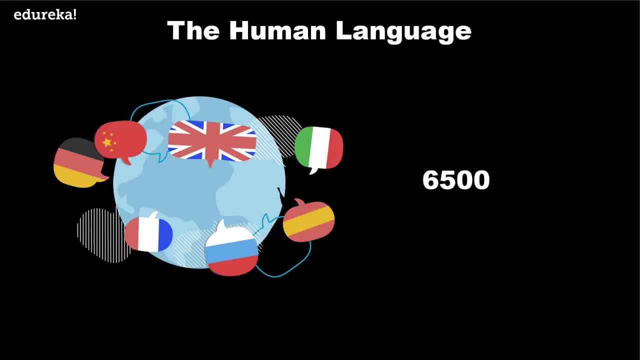 The human language is a mystery, with over 6,500 languages worldwide. When a language contains words that are derived from another word as their use in the speech changes, it's called inflected language. Now, almost all the languages have this feature and most of them are inflected language. According to industry estimates, only 21%. 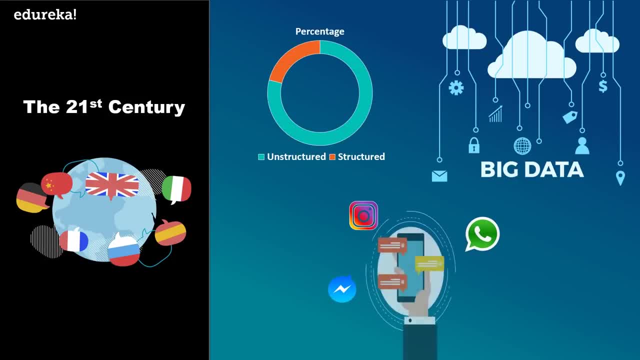 of the available data is present in structured form. Data is being generated as we speak, as we tweet, as we send messages on WhatsApp or Instagram or iMessaging and in various other activities. Now, majority of this data exists in the textual form, which is highly unstructured. 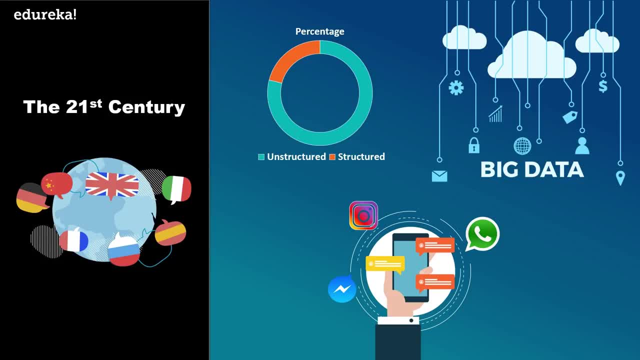 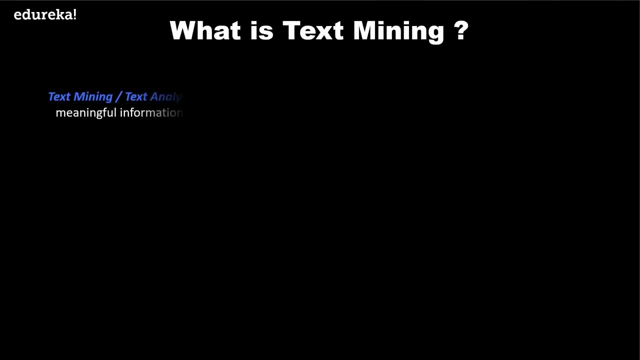 Now, in order to produce significant and actionable insights from text data, it is important to get acquainted with the techniques and principles of text mining and natural language processing. So let's understand these terms. So let's begin with text mining. Text mining or text analytics is the process of deriving meaningful information. 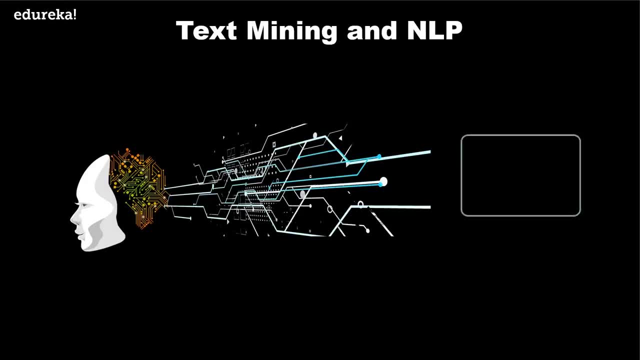 from natural language text, As text mining refers to the process of deriving high quality information from the text. So let's begin with text mining. Text mining refers to the process of deriving high quality information from the text. Now the overall goal is essentially to turn text. 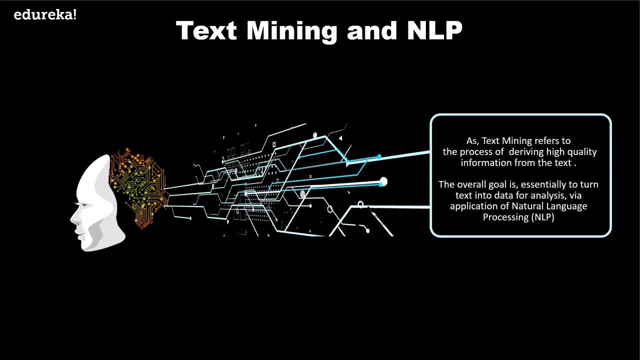 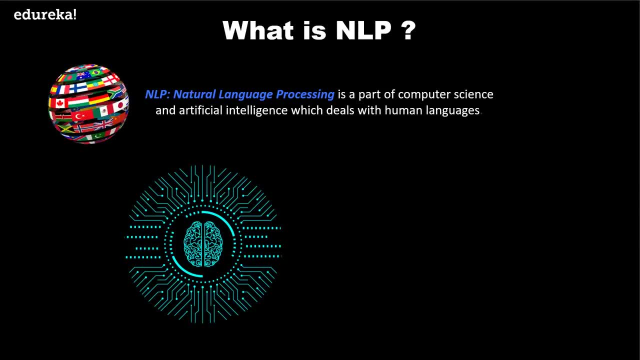 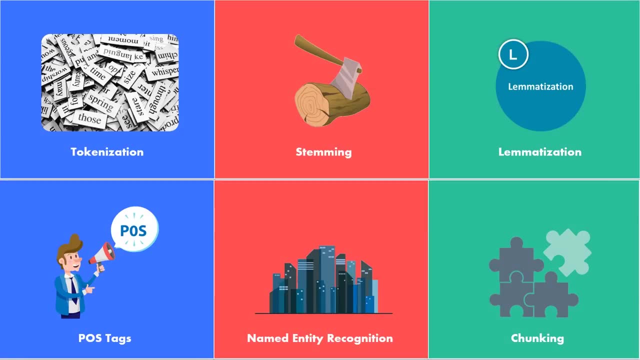 into data for analysis via application of natural language processing. Now, natural language processing refers to AI method of communicating with an intelligent systems using a natural language. So here are the different steps involved in the process of NLP. So we have tokenization, stemming, lemmatization, POS tags, named entity recognition and chunking. 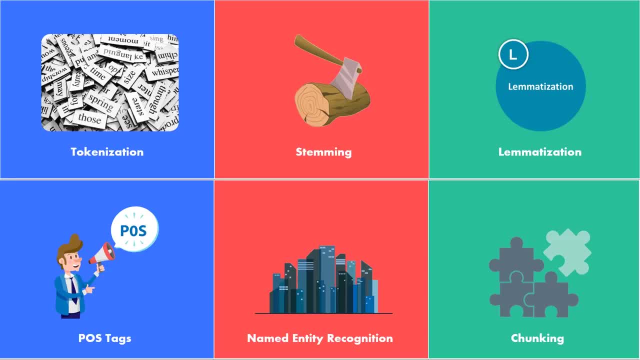 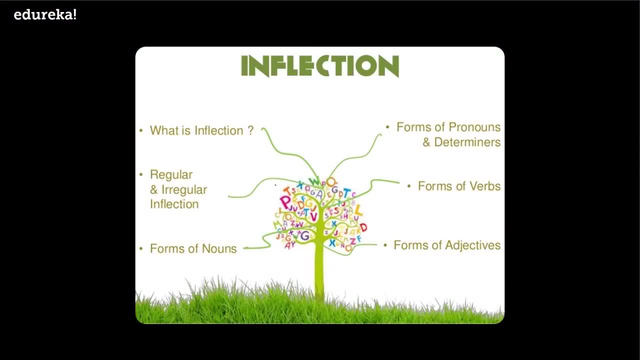 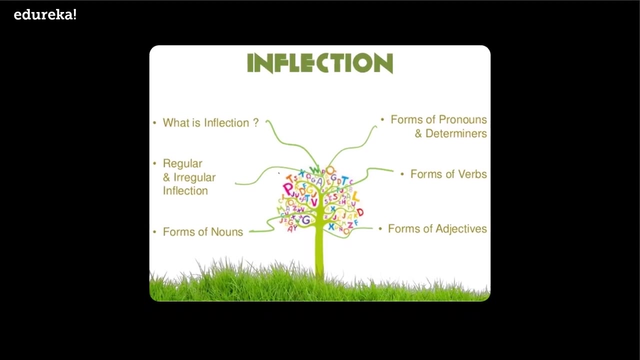 So today our focus will be on stemming and lemmatization. Now, the degree of inflection may be higher or lower in a language. As you have read the definition of inflection with respect to grammar, you can understand that an inflected word will have a common root form: Stemming- and 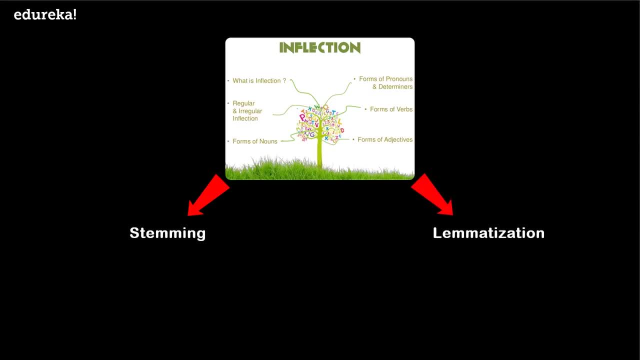 lemmatization have been studied and algorithms have been developed in computer science since the 1960s. In this video, you will learn about stemming and lemmatization in a practical approach, covering the background, some famous algorithms, applications of stemming and 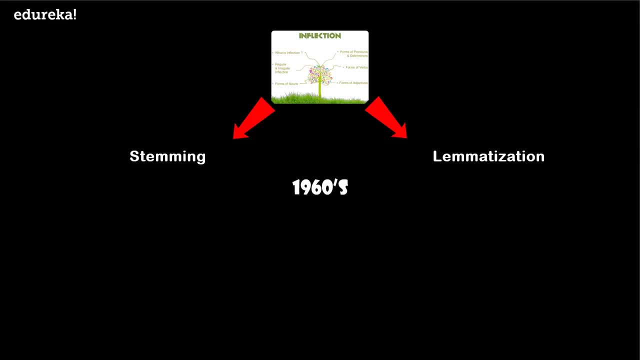 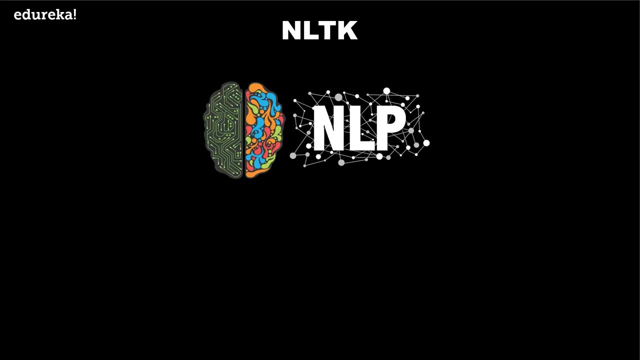 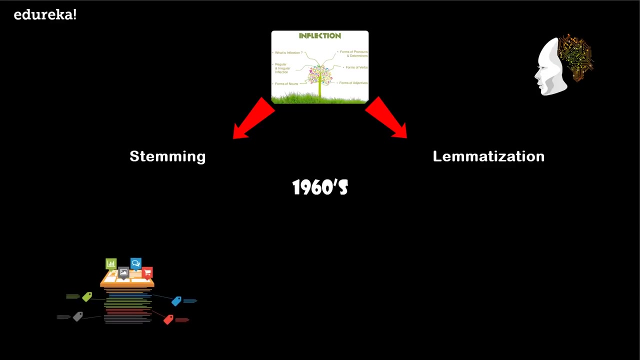 lemmatization and how to stem and lemmatize words, sentences and documents using the Python NLTK package, which is the natural language toolkit package provided by Python for natural language processing tasks. Now, stemming and lemmatization are text normalization techniques. 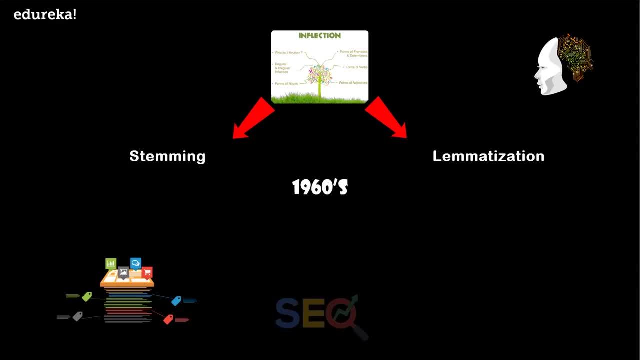 in the field of natural language processing that are used to prepare text, words and documents for the language processing process. So let's get started. So stemming and lemmatization are text normalization techniques that are used to prepare text, words and documents for further processing, And these are widely used in tagging systems, indexing SEO. 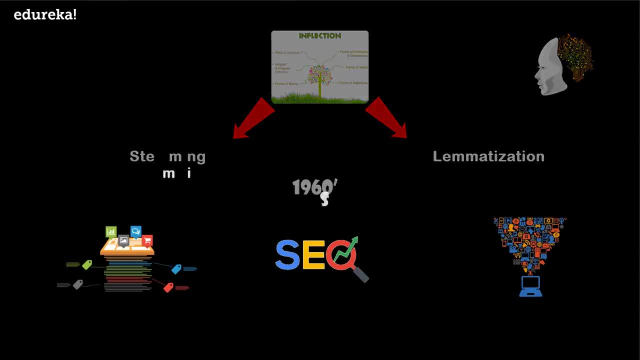 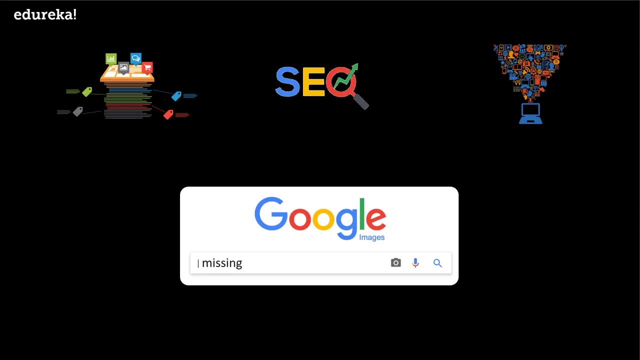 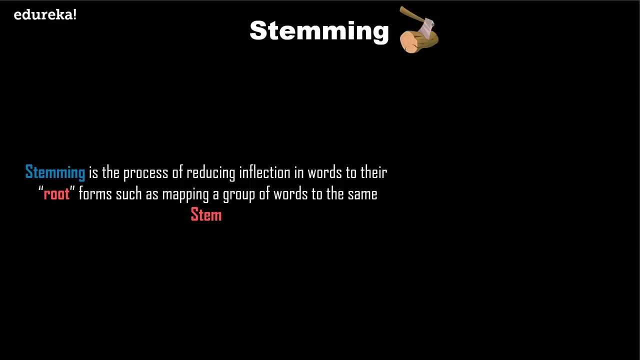 web search results and information retrieval Now, for example, searching for the word miss on Google will also result in Mrs Missing, as miss is basically the stem of both these words. So let's start with stemming Now. stemming is the process of reducing inflection in words to 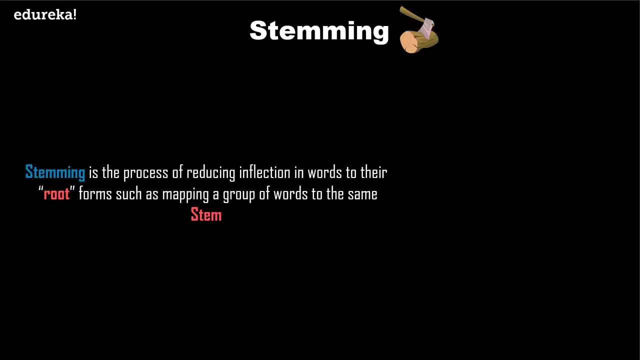 their root forms, such as mapping a group of words to the same stem, even if the stem itself is not a valid word in the language. Now there are English and non-English stemmers available in NLTK package. Now for the English language, you can choose: 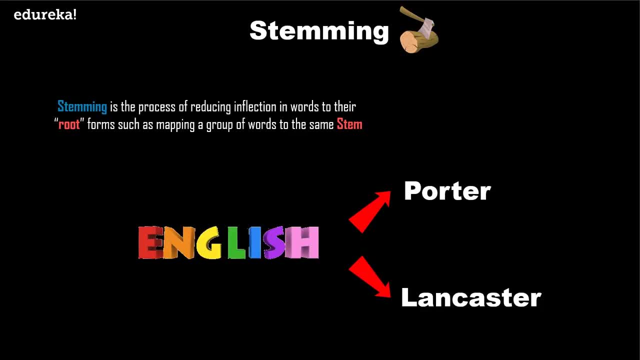 between Porter stemmer and Lancaster stemmer, Porter stemmer being the oldest one, originally developed in 1979.. Lancaster stemmer was developed in 1990 and uses a more aggressive approach than Porter stemming algorithm. So let's try out the Porter stemmer to stem words And along with it. 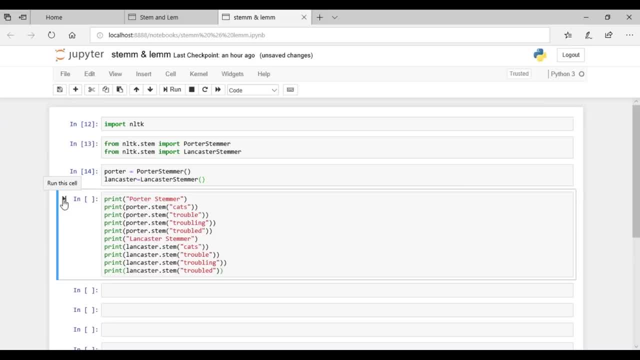 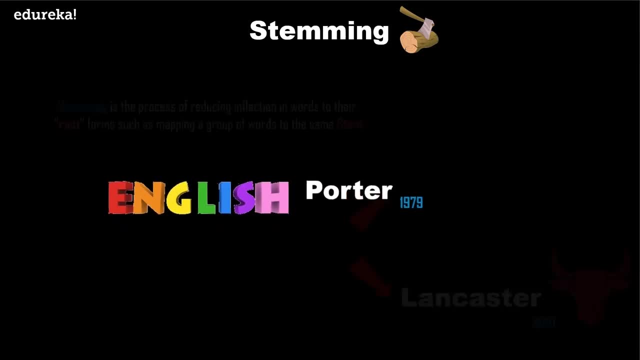 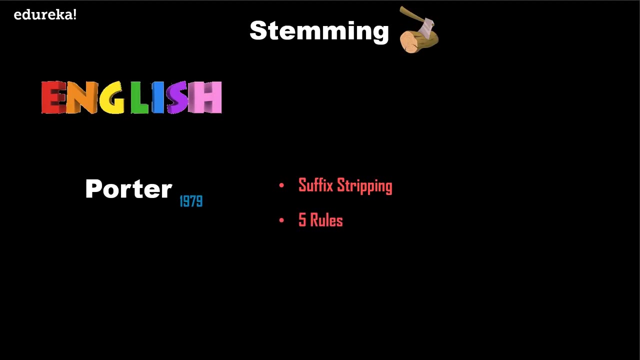 you will see how it is stemming the words. So this is how the code for Porter stemmer works. Now Porter stemmer uses suffix stripping to produce stems. Porter stemmer algorithm does not follow linguistics, rather a set of five rules for different cases that are applied in phases to. 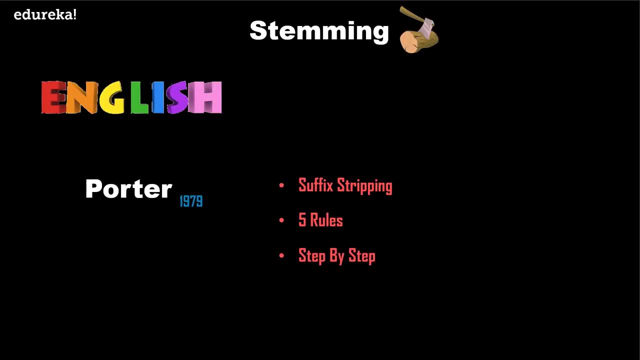 generate stems. Now, this is the reason why Porter stemmer does not often generate stems that are actual English words. Now, it does not keep a lookup table for actual stems of the word, but it that applies algorithmic rules to generate stems. 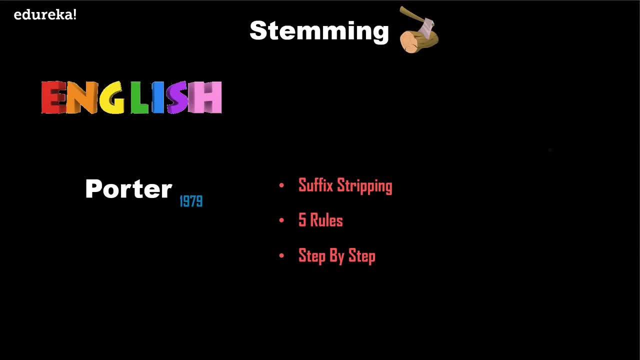 It also uses the rules to decide whether it is wise to strip a suffix. Now one can generate its own set of rules for any language. That is why Python NLTK introduced snowball stemmers that are used to create non-English stemmers. 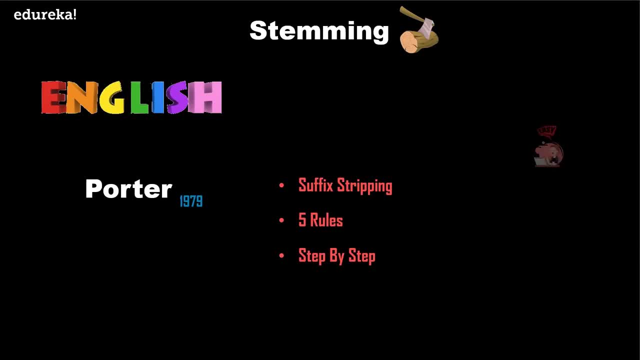 So why do we use it Now? PortaStemmer is known for its simplicity and speed. It is commonly useful in information retrieval environments, known as IR environments, for fast recall and fetching of search queries, such as for words like connections, connected, connecting or connection. 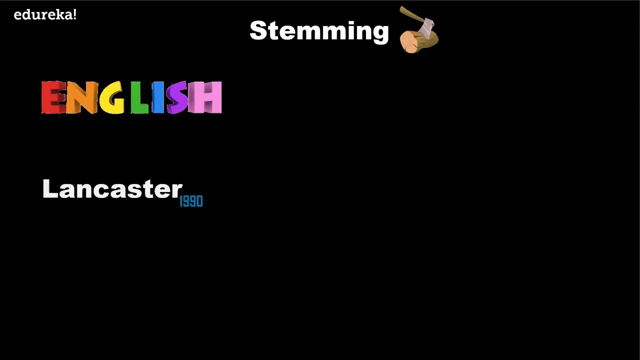 All of these words mean connect. Now, the Lancaster stemmer is an iterative algorithm with rules saved externally. Lancaster stemmer is simple but heavy stemming due to iterations, and overstemming may occur. Now, overstemming causes the stems to be not linguistic or they may have no meaning at all. 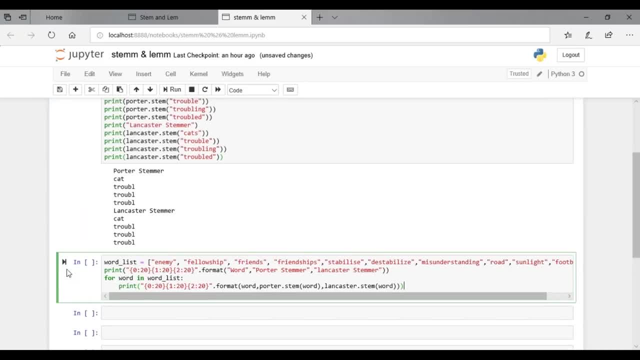 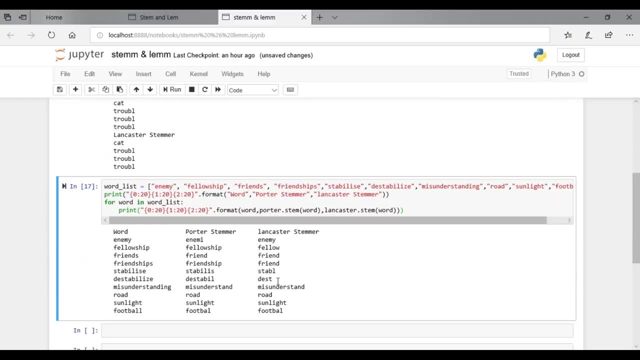 So now let's have a look at the Lancaster stemmer code, For example. in above code destabilized is stemmed to dest in Lancaster stemmer, whereas using PortaStemmer, destable Now Lancaster stemmer produces an even shorter stem than Porta because of iterations and overstemming is occurred. 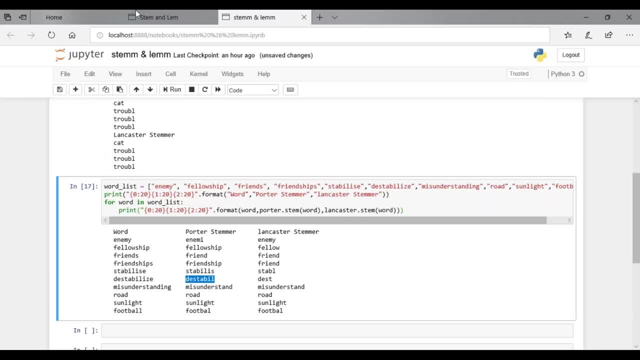 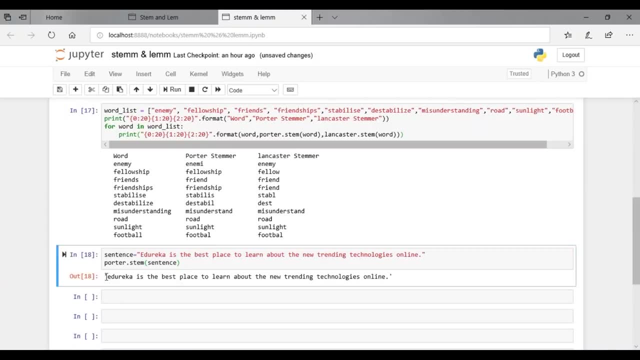 So you can stem sentences and documents using NLTK stemmers using the following code: So, as you see, the stemmer sees the entire sentence as a word, so it runs it as it is. Now we need to stem each word in the sentence and return a combined sentence. 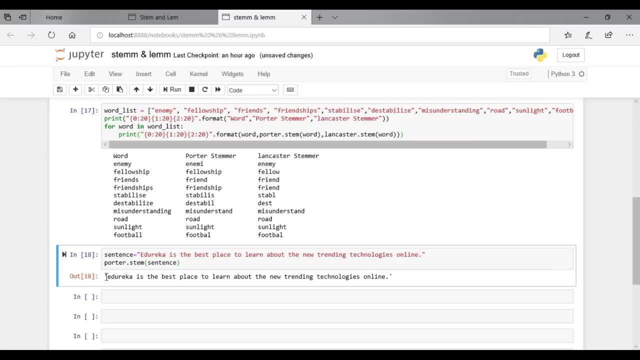 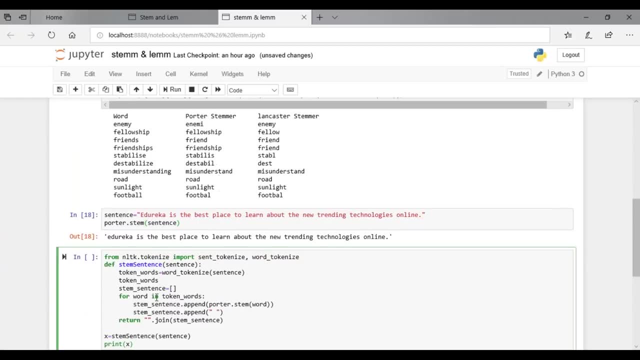 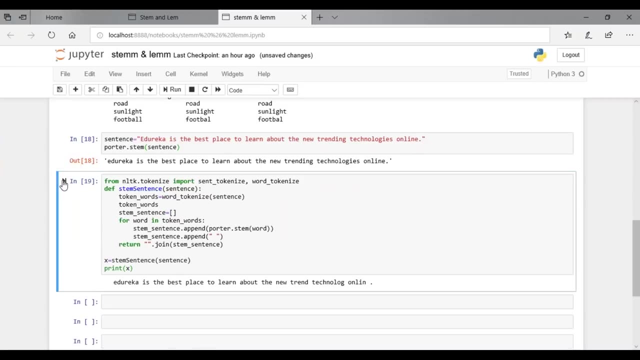 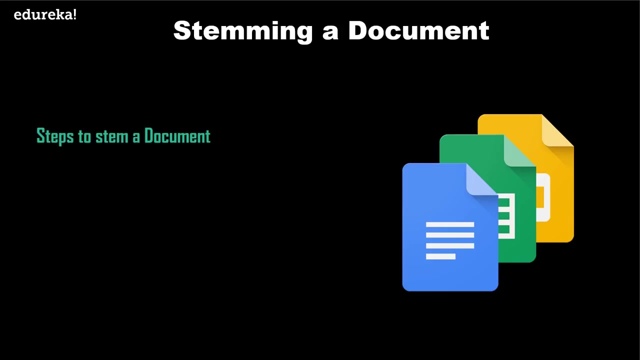 Now to separate the sentence into words, you can use tokenizer. The NLTK tokenizer separates the sentence into words. So let's see how it's done. Now, to stem a document, we need to do the following steps. first, We have to take a document as the input. next, 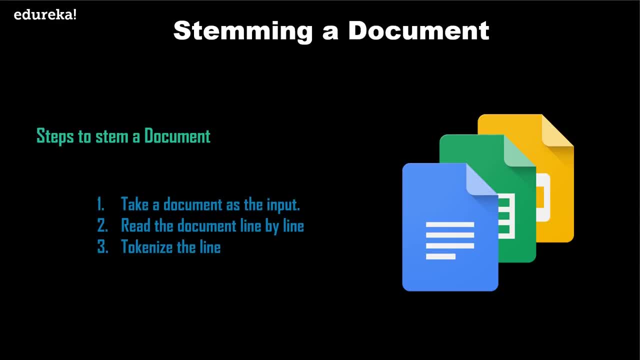 We have to read the document line by line and then tokenize the line. next we have to stem the words and finally we will output the stemmed words. So let's do some coding. now open a file. that is any text file. So I have a text file named deep learning. 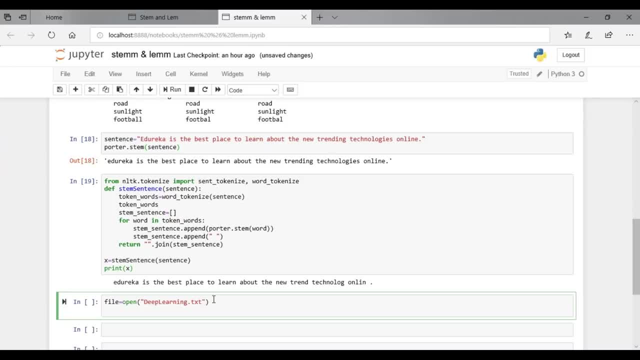 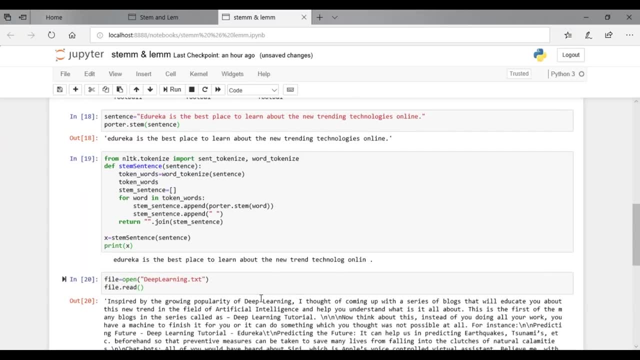 and you have to provide your complete file path in open command of python if it is stored in any other directory. now you can see the content of the file using the dot read method. all together, Now you can maintain the lines in a file in a python list. 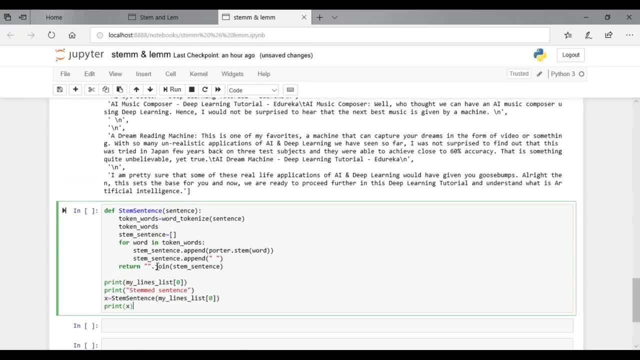 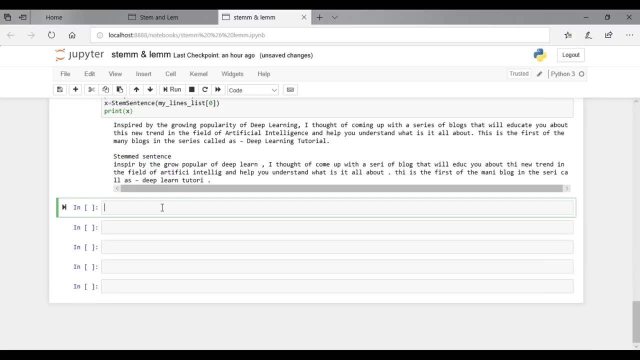 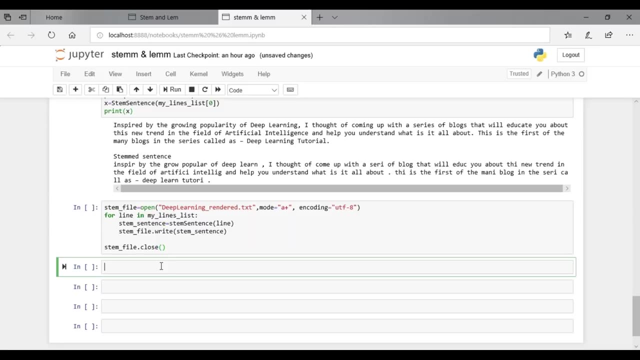 using read lines method. You can now access each line and use the tokenize- stem sentence function that you created before to tokenize and stem the line. Now you can save the stemmed sentence to a text file using python write lines function. make a list first to store all. 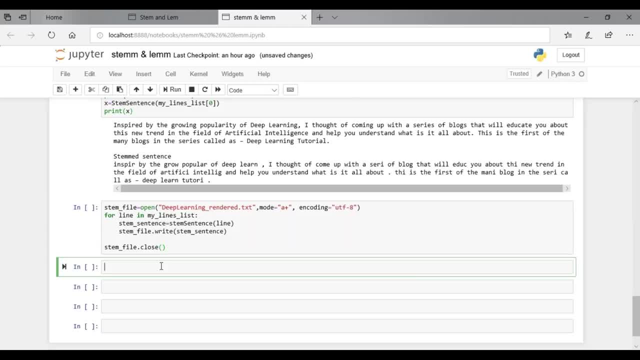 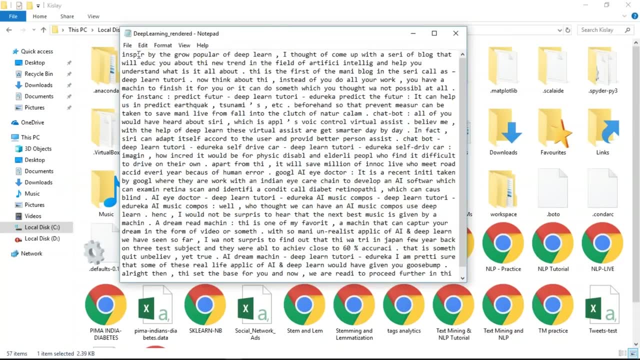 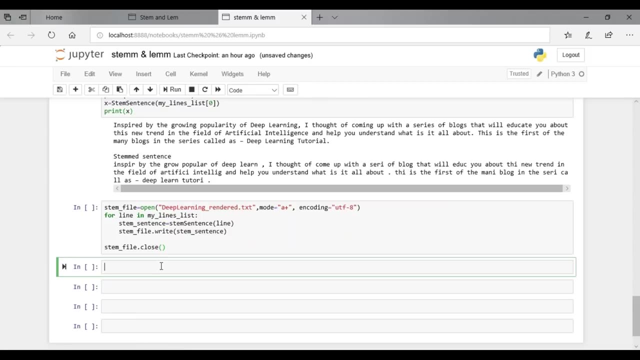 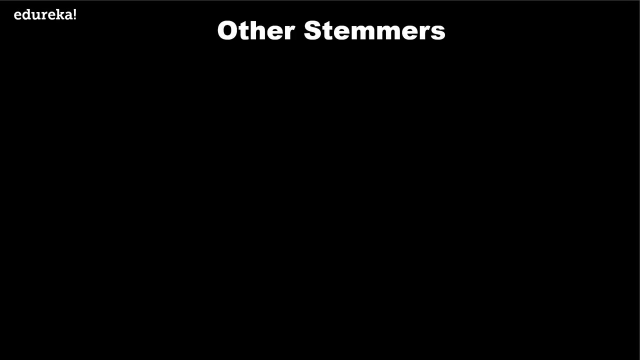 the stemmed sentences and simply write the list to the file Using write line. So the text file created will be as follows: Python NLTK provides not only to English stemmers, that is, Porter stemmer and Lancaster stemmer, but also a lot of non-english stemmers as part of snowball. 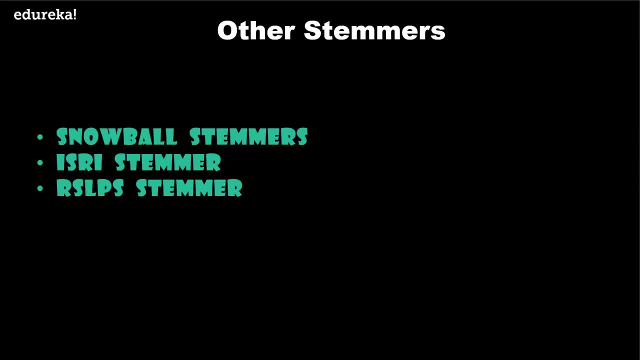 stemmers is RI stemmer, RSLP a stemmer. now python NLTK included snowball stemmers as a language to create non-english stemmers. currently it supports the following languages: Danish, Dutch, English, French, German and much more. now lemmatization- unlike stemming- reduces. 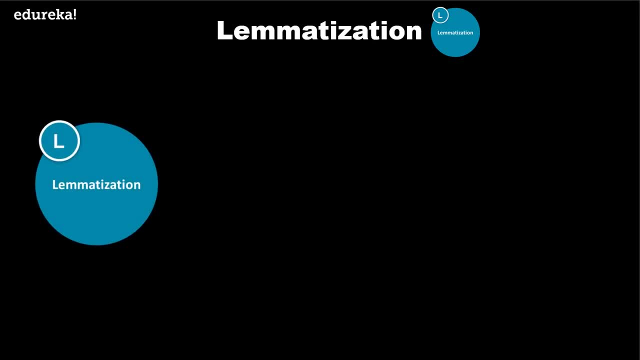 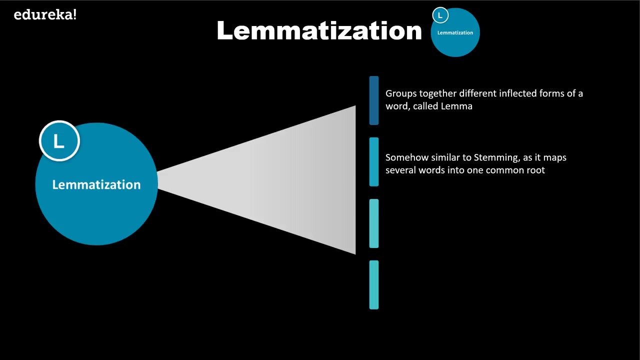 the inflected words, properly ensuring that the root word belongs to the language. in lemmatization, root word is called lemma. lemma is the canonical form, dictionary form or the citation form of a set of words. Now it takes into consideration the morphological analysis of 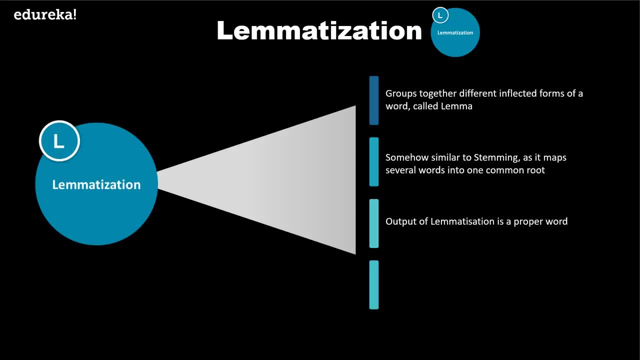 the words. to do so it is necessary to have detailed dictionaries which the algorithm can look through to link the form back to its lemma. For example, a lemmatizer should map gone going and went into go now. python NLTK provides word net lemmatizer that uses the 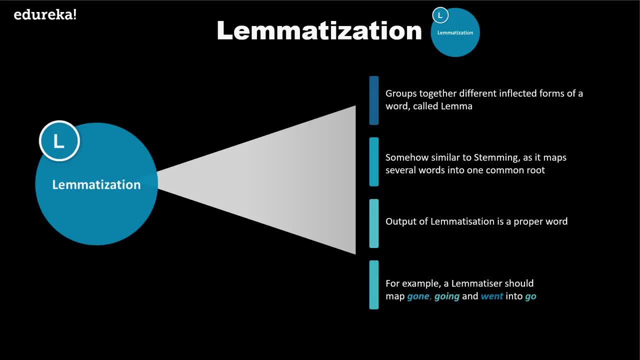 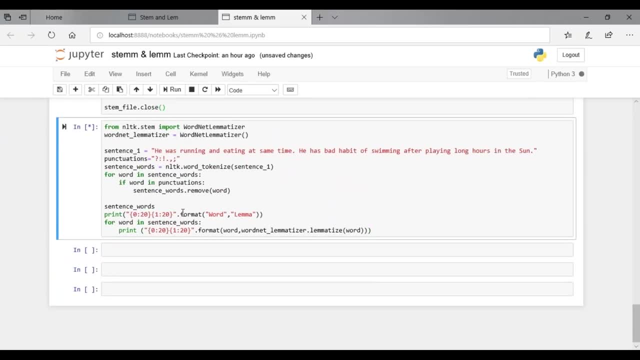 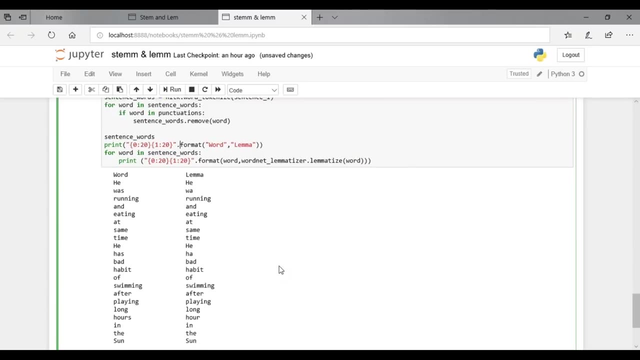 word net database to look up lemmas of words. So let's have a look at the code Now. in the above output, you must be wondering that no actual root form has been given for any word. This is because they are given without context. now you need. 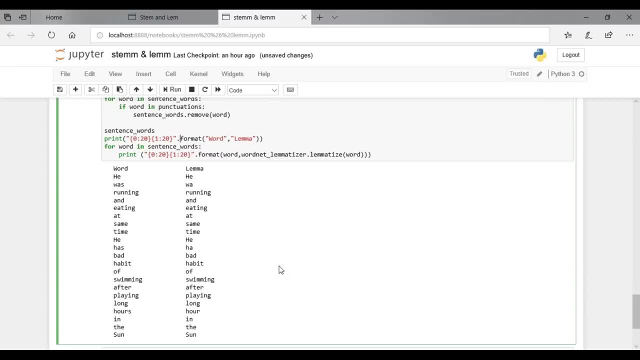 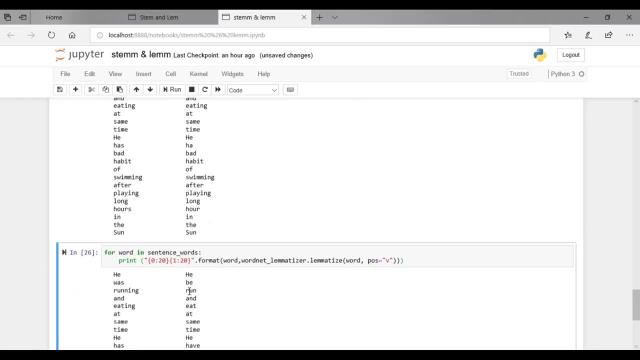 to provide the context in which you want to lemmatize. that is, the parts of speech. Remember when we were learning about the different steps in NLP, POS tag was an important step in the whole process. Now this is done by giving the value for POS parameter in word. 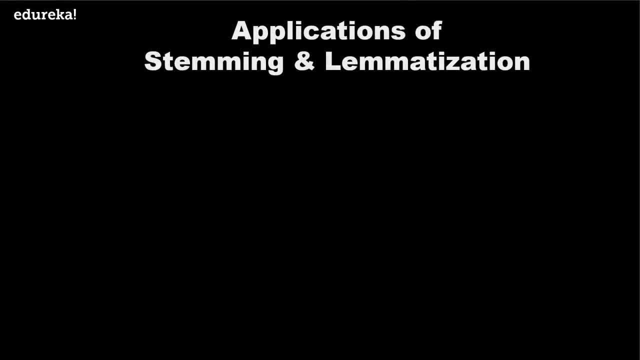 net lemmatizer dot lemmatize. So let's have a look at some of the applications of stemming and lemmatization. The first one is sentiment analysis. now, sentiment analysis is the analysis of people's reviews and comments about something. it is widely used for analysis of products on online retail shops. 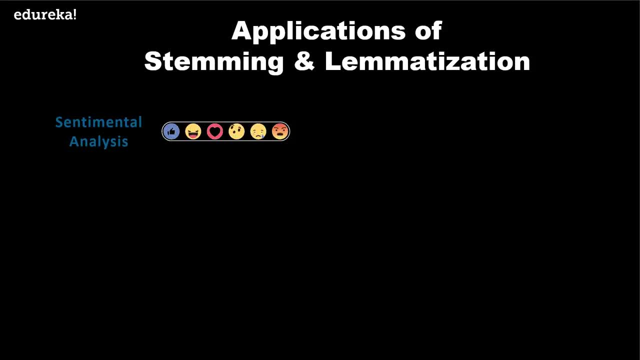 Now stemming and lemmatization is used as part of the text preparation process before It is Analyzed. next up is document clustering. Now, document clustering is the application of cluster analysis to textual documents. It has applications in an automatic document organization, topic extraction and fast information retrieval or filtering. 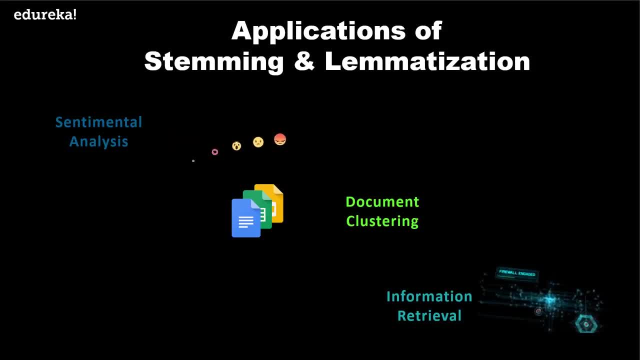 next one is information retrieval environments. Now it is useful to use stemming and lemmatization to map documents to common topics and display search results by indexing when documents are increasing to mind-boggling numbers. Now you may be asking yourself: when should I use stemming and 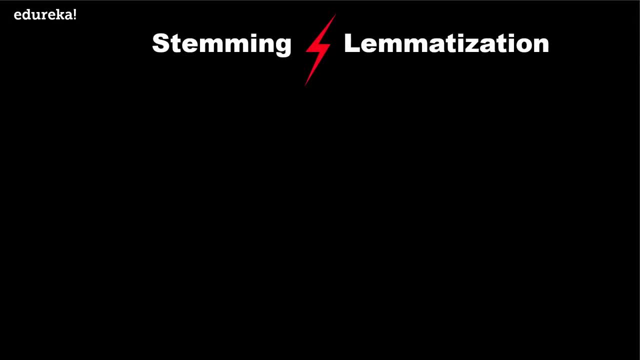 when should I use lemmatization? now? stemming and lemmatization both generate the root form of the inflected words. The difference is that stem might not be an actual word, Whereas lemma is an actual language word. now, stemming follows an algorithm with steps to perform on the words, which makes 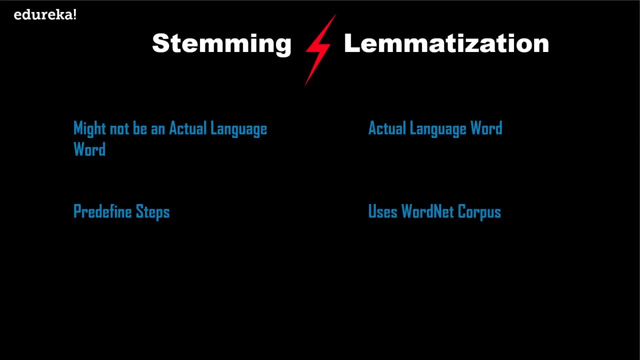 it faster, Whereas in lemmatization You use wordnet corpus and a corpus for stop words as well to produce lemma, which makes it slower than stemming. You also have to define a parts of speech to obtain the correct lemma. So when to use what now? the above points show that if speed is